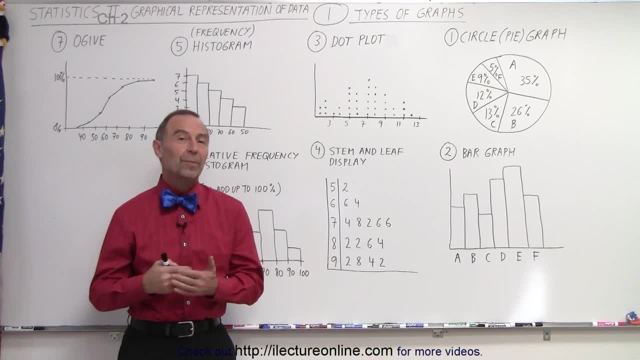 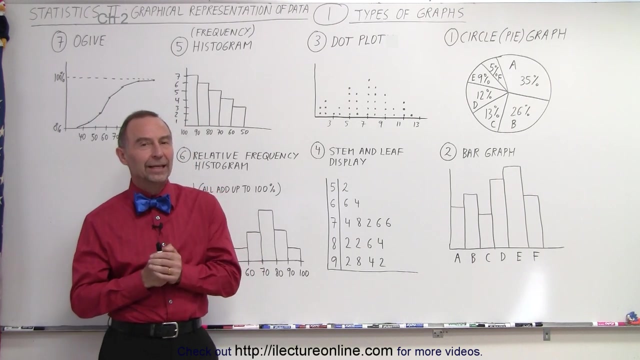 Welcome to iLecture Online. The second chapter in statistics is dealing with graphical representation of data. Well, it's collecting data, organizing them, graphing them and then interpreting those graphs. There's a lot of work to be done in this chapter and it all surrounds specific ways in 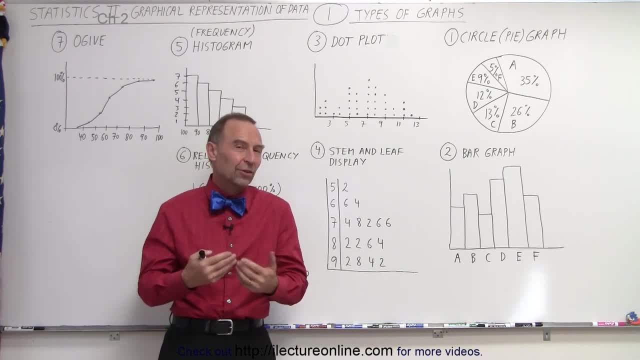 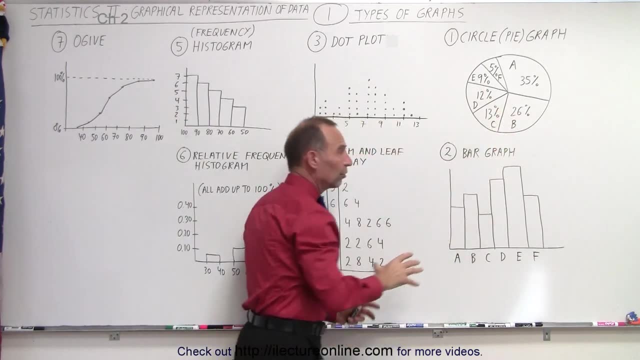 which we can represent the data. So here are some of the ways, some of the graphs that we will encounter in this chapter. First of all, we'll be encountering the circle graph, or also called the pie graph. So you can see that each slice of the pie represents a certain input of the data and you 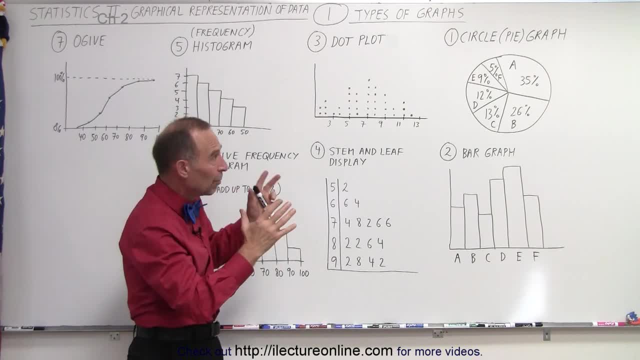 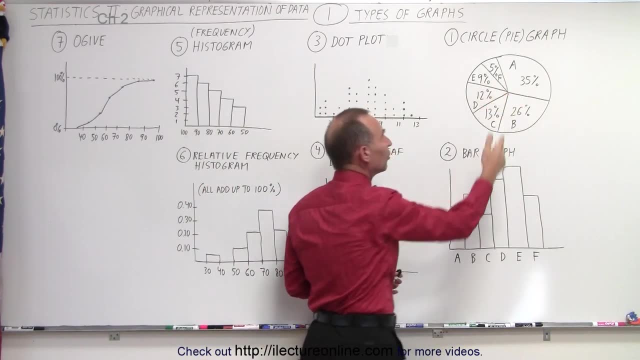 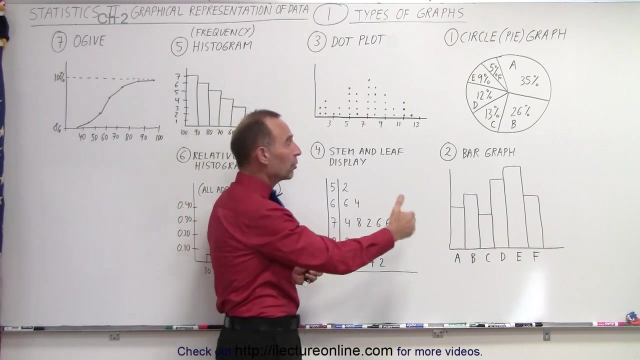 can see that typically the larger size of the pie means that more of it belongs to that specific data type. So here we have it generally labeled A, B, C, D, E, F, and you can see the relative percentages that each of those data types represent. Instead of the circle graph, sometimes we use the bar graph. 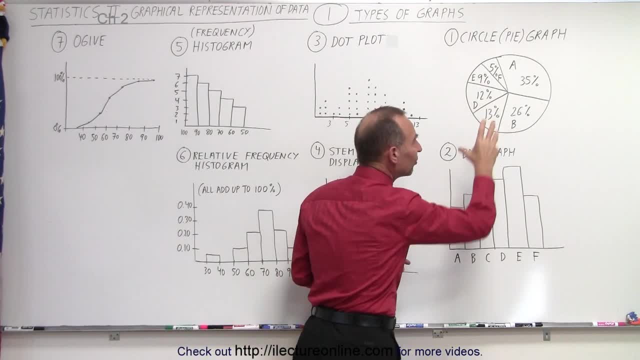 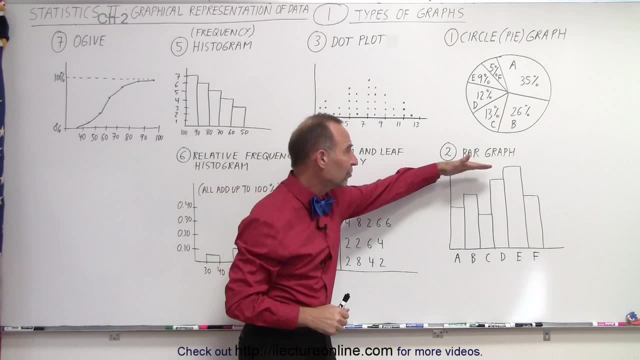 The bar graph gives you much more of a relative height. The sizes, especially when there's a lot of slices, are more important, So you can see that each slice of the pie represents a certain input of the data. The sizes in the pie make it sometimes difficult to see if one is bigger than the other. With bar graphs you can. 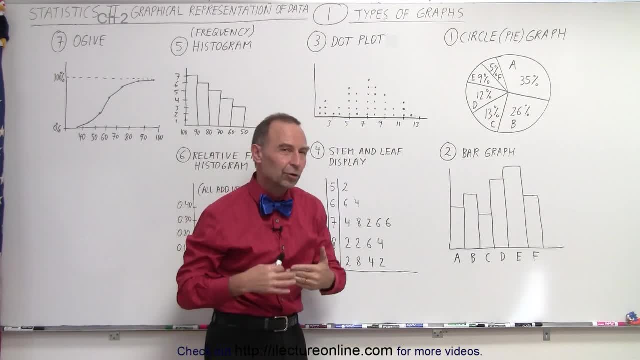 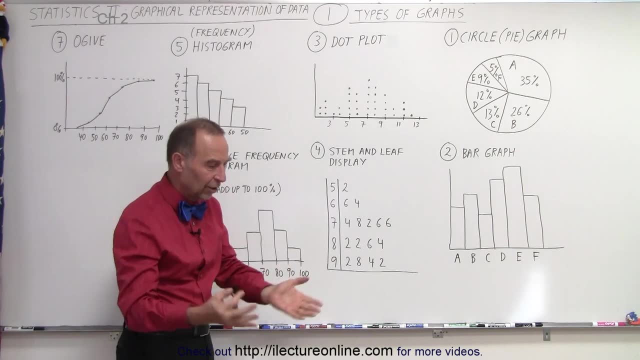 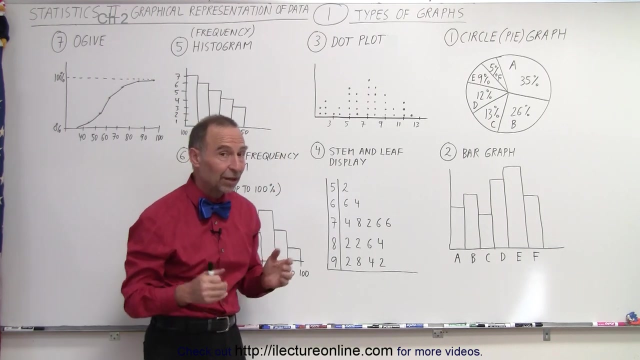 actually see very quickly which ones have the greatest height and therefore the greatest representation in the data set. We'll also encounter dot plots, which are very handy when you have a random set of data that you want to graph quickly. We'll talk about the stem and leaf display, which has some interesting aspects of it as well. 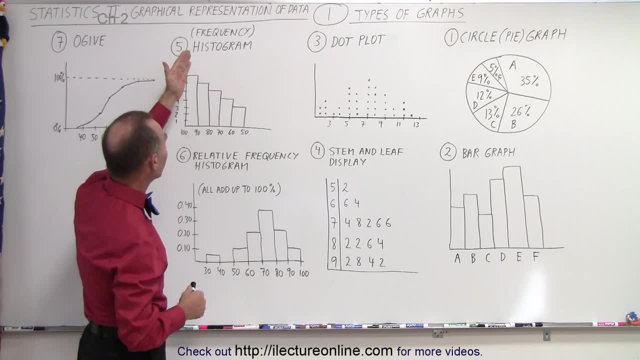 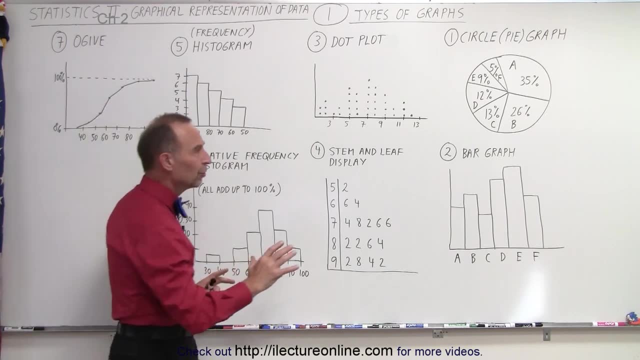 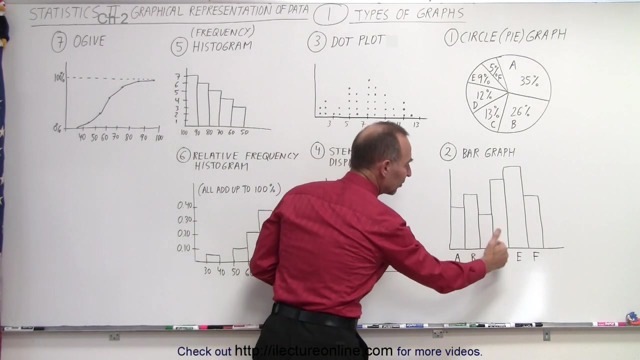 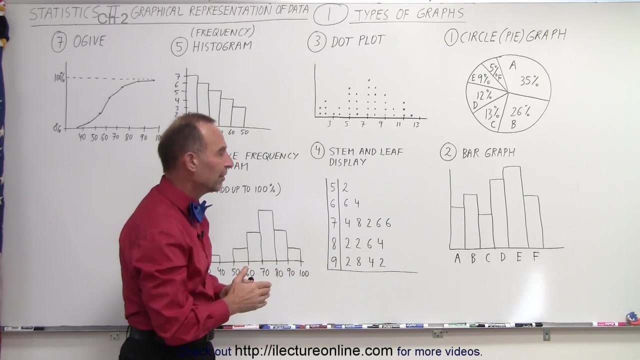 We'll also talk about the histogram. We have what we call the frequency histogram. A lot of times people get confused between the difference between bar graphs and histograms. Typically, bar graphs are associated with specific data sets. For example, if you have the number of types of cars, there's only one type of car of that type, and so you want to then see how many you have of each type. 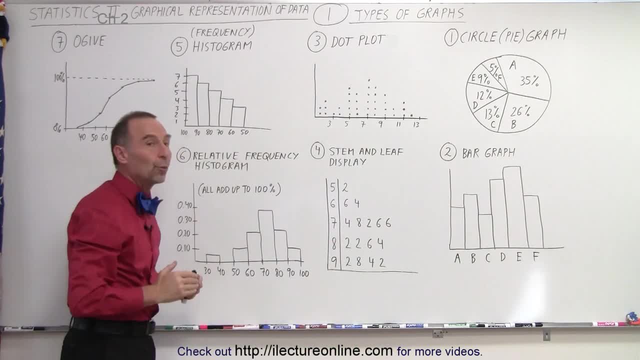 Where in a histogram you typically talk about data over a range. so anything between 90 and 100 fits in This data type. between 80 and 90 fits in this data type, but we'll get into the differences in a little bit more detail.